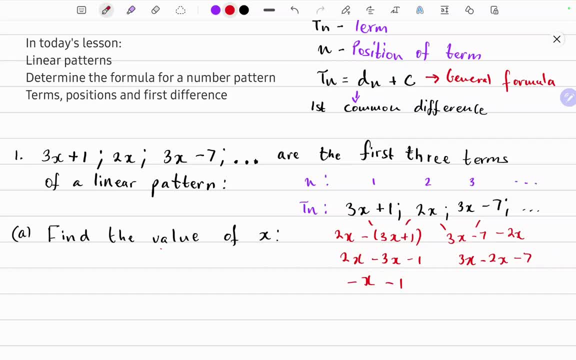 So here we should get minus x minus 1.. And here we have x minus 7.. So we can replace these with the simplified versions. So the first difference here is minus x minus 1. And here is x minus 7.. I'm going to reiterate the first difference, for a linear pattern is a constant. 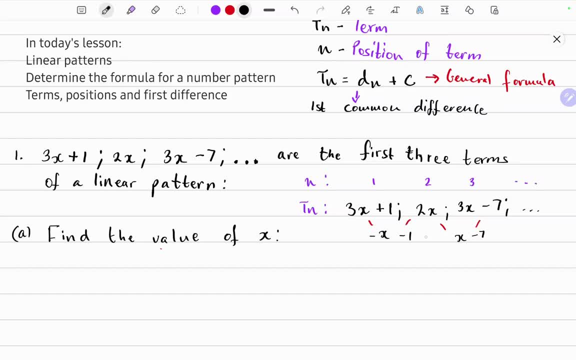 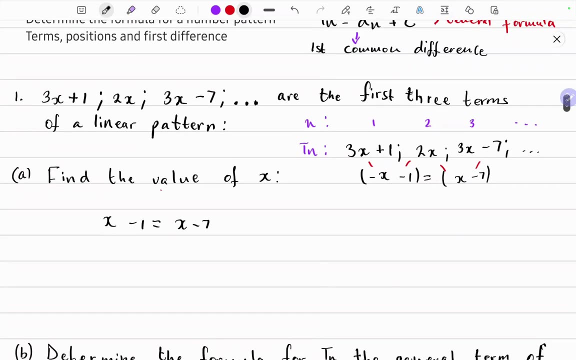 And because it's a constant, you can equate these two, Because they are equal, So we can find x. So therefore x minus 1 should be equal to x minus 7.. So here, if you collect like terms, you should get: minus 2x is equal to negative 6.. 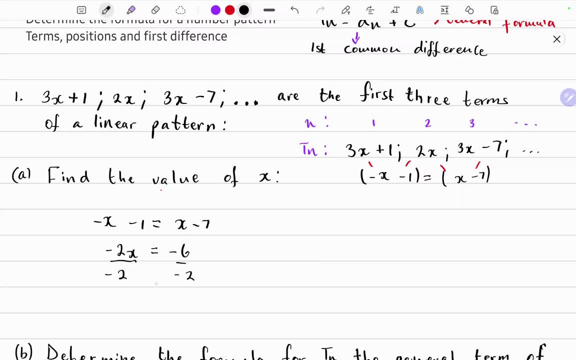 Divide both sides by negative 2. Which would give us x is equal to Positive 3. So now we can substitute: 3. To get the constant difference in a numeric format. So negative 3 minus 1 is negative 4.. 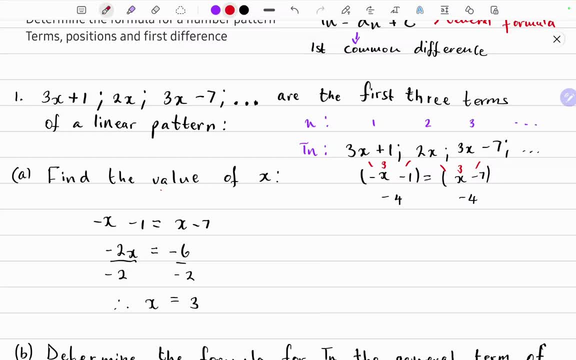 And 3 minus 7 is negative 4.. So the constant difference for this number pattern D is equal to negative 4.. And we can substitute 3 in each of these To get this number pattern in a numeric format. So after substituting we get: 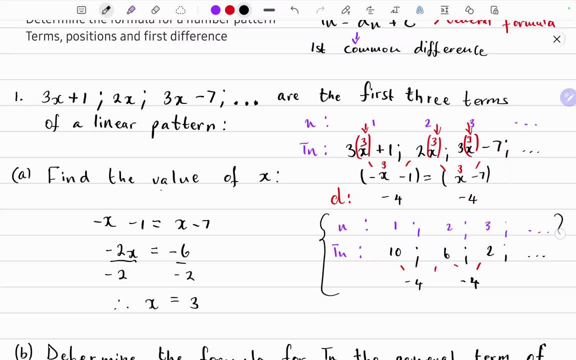 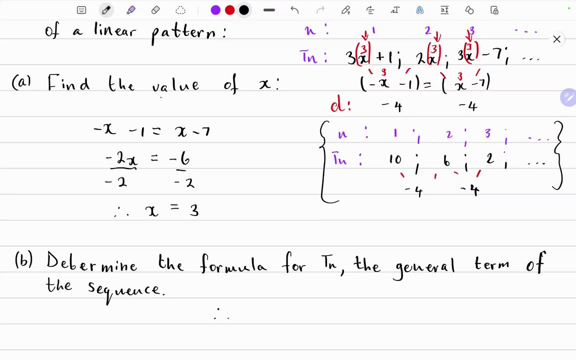 So this is the number pattern we get after substituting x in its respective places. So equation B says: determine the formula for Tn, the general term of the sequence. A good place to start is to write the general formula for any linear pattern, that is: tn is equals to dn plus c, where d is the constant the first. 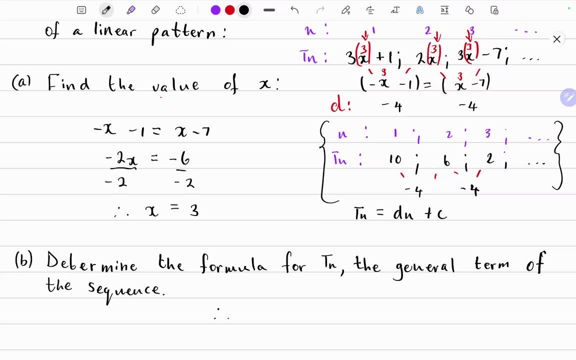 constant difference: tn is the term, n is the position of that term and c is just the constant. so we can substitute information that we have to find the formula for this pattern. so tn is equals to d. the constant difference is minus four. first constant difference, n plus c. 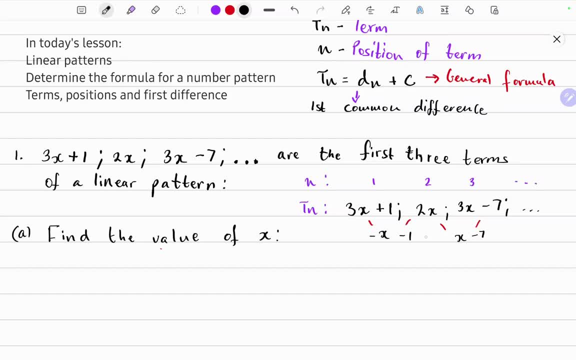 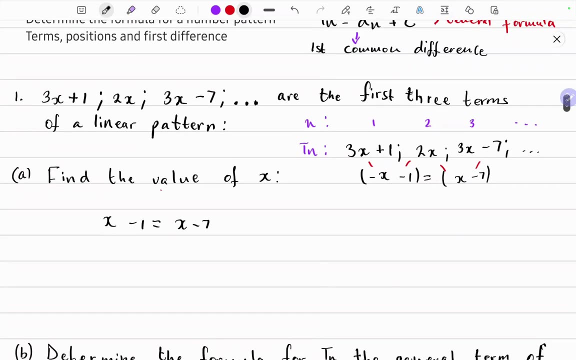 And because it's a constant, you can equate these two, Because they are equal, So we can find x. So therefore x minus 1 should be equal to x minus 7.. So here, if you collect like terms, you should get: minus 2x is equal to negative 6.. 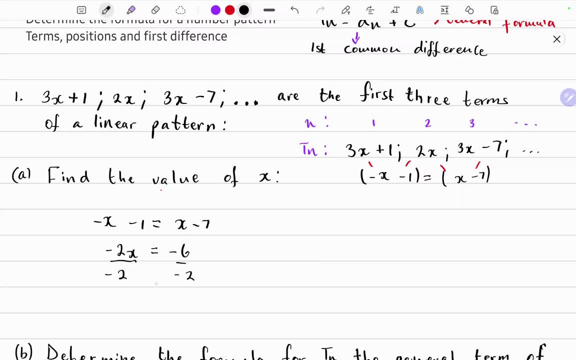 Divide both sides by negative 2. Which would give us x is equal to Positive 3. So now we can substitute: 3. To get the constant difference in a numeric format. So negative 3 minus 1 is negative 4.. 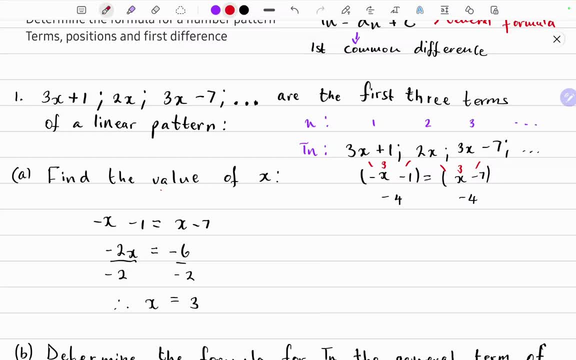 And 3 minus 7 is negative 4.. So the constant difference for this number pattern D is equal to negative 4.. And we can substitute 3 in each of these To get this number pattern in a numeric format. So after substituting we get: 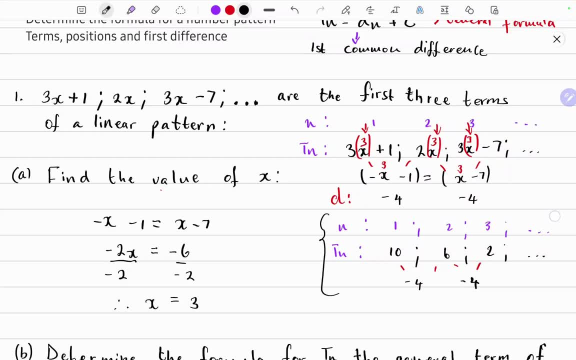 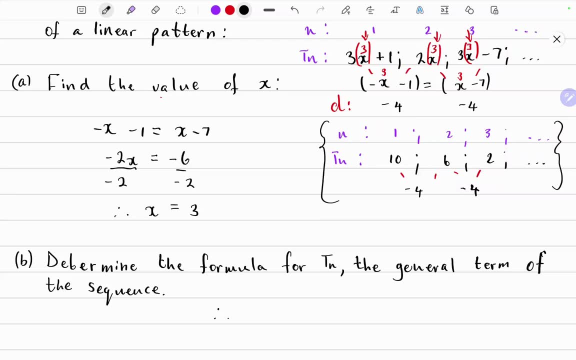 So this is the number pattern we get after substituting x in its respective places. So question B says: determine the formula for tn, the general term of the sequence. A good place to start is to write the general formula for n linear pattern, that is: TN is equals to DN plus C, where D is the constant the. 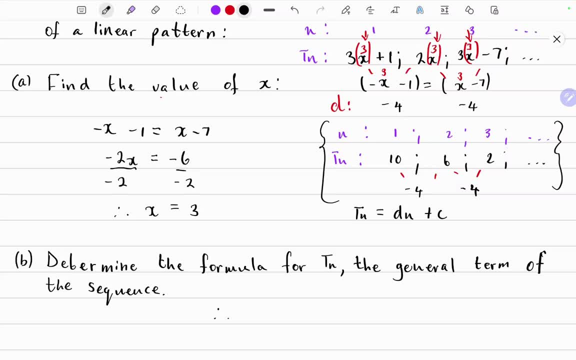 first constant difference: TN is the term, N is the position of that term and C is just the constant. so we can substitute information that we have to find the formula for this pattern. so TN is equals to D. the constant difference is minus 4. first constant difference: N plus C. it's possible to find C by using any pair of.